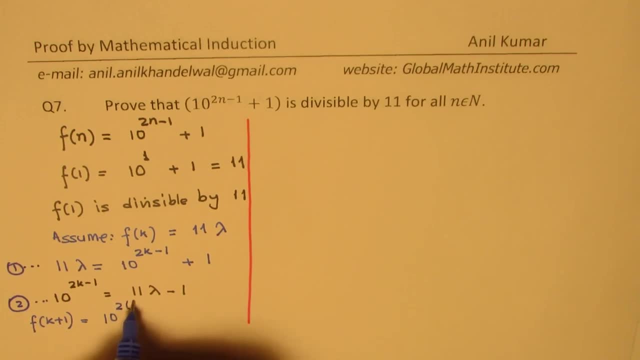 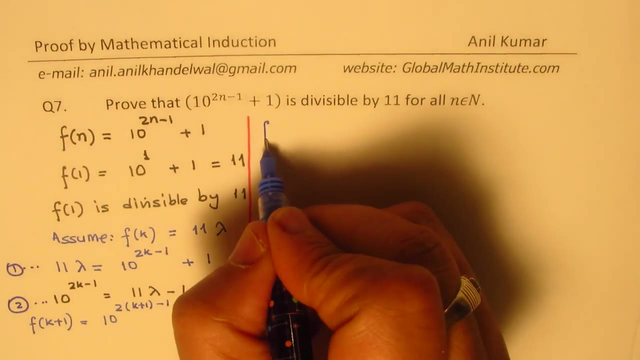 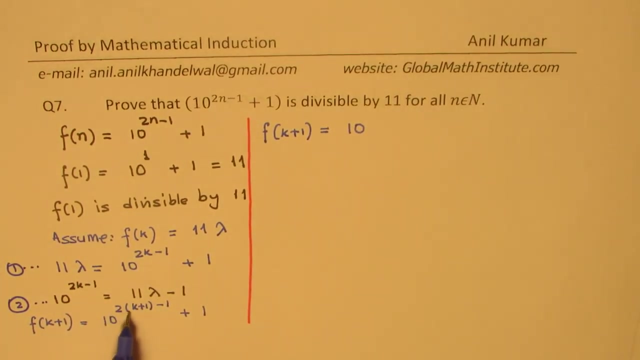 10 to the power of 2 times k plus 1 minus 1 plus 1, correct. So let's take it to the right side and simplify. So f of k plus 1 is indeed equals to 10 to the power of 2k plus 2, so we can write this as 2k minus 1 plus 2, right. 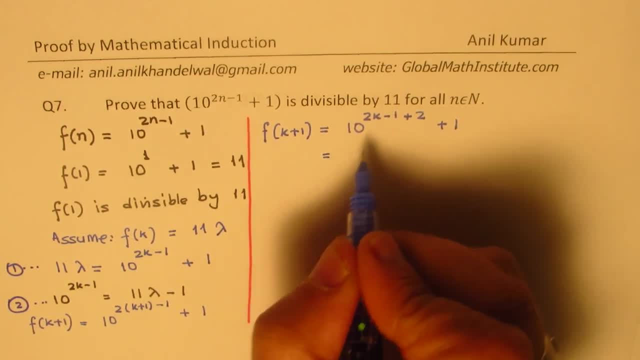 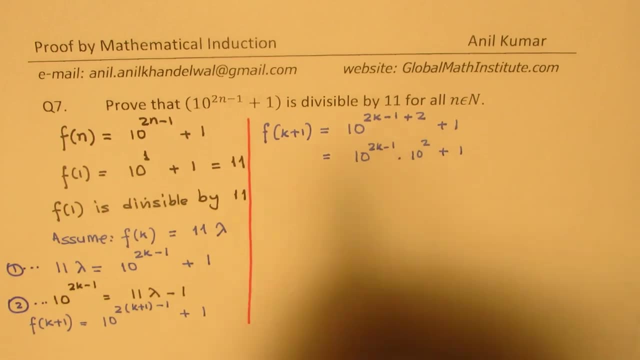 I'm just rearranging So which you could write here as 10 to the power of 2k, k minus 1 times 10 to the power of 2 plus 1, right Now we rearrange and wrote 10 to the. 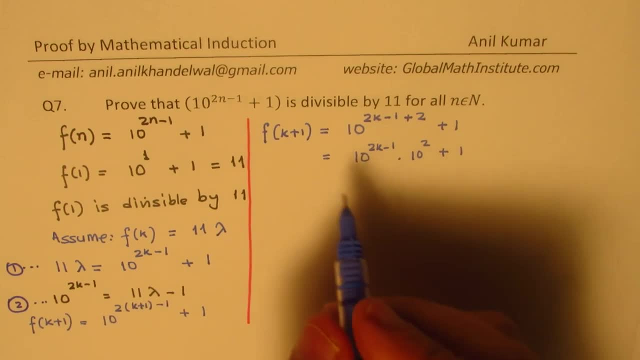 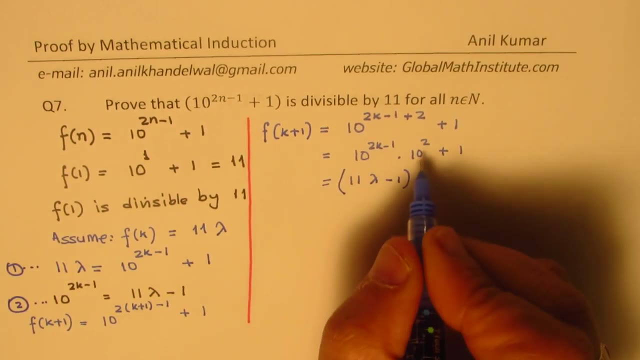 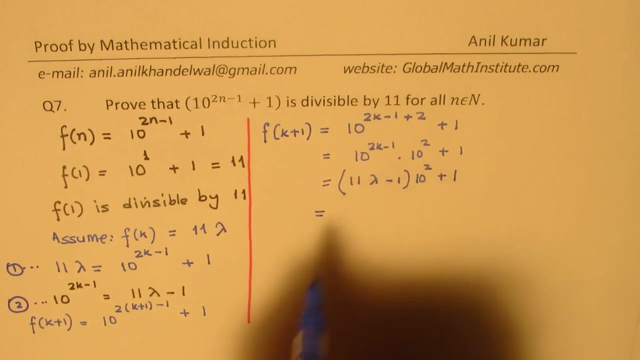 power of 2 k minus 1 as 11 lambda minus 1.. So I could write this as 11 lambda minus 1 times 10 square, which is 100 plus 1.. So that is 100, right, So we can now open this bracket. 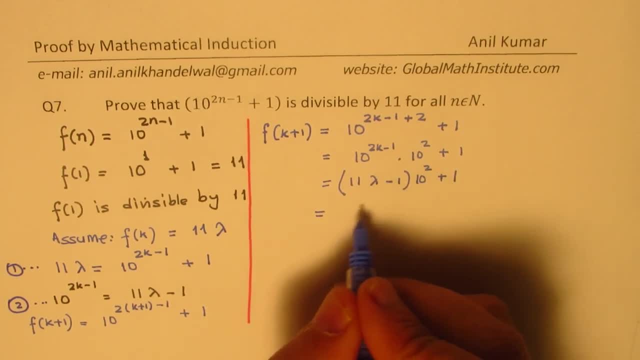 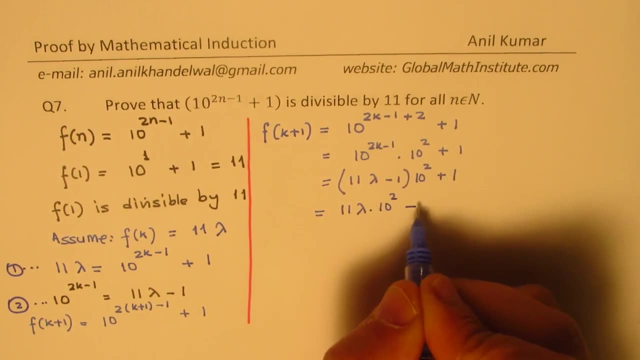 so once you open this bracket, what do you get? You get 11 lambda times: 10 square minus 10 square plus 1.. Now 10 square is 100.. So 101 is 99.. So what we get here is 11 lambda times. let us write. 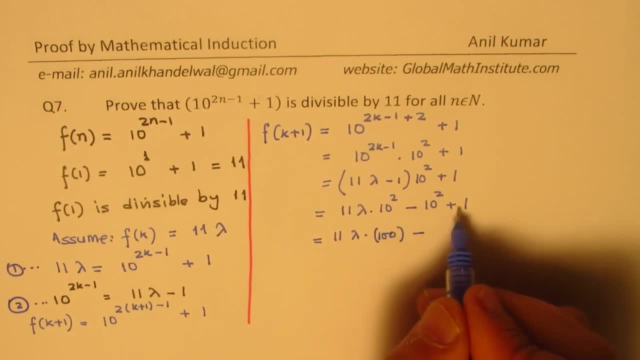 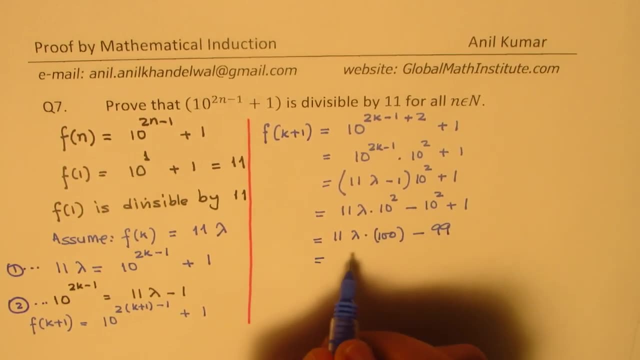 this as 100 minus, That is 99, right, 100 plus minus 100 plus 1, and from here 11 is a common factor. So taking 11 as a common factor, we get 100 lambda minus 9.. So clearly, f of k plus 1 is a multiple. 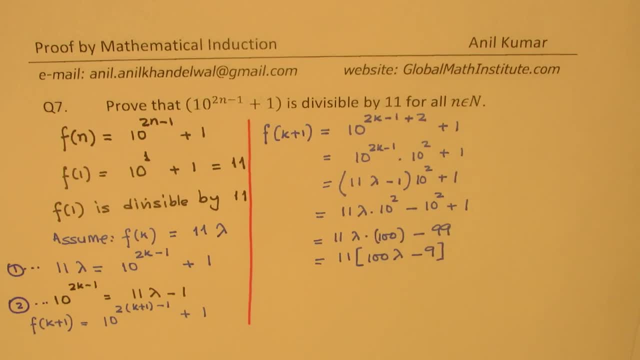 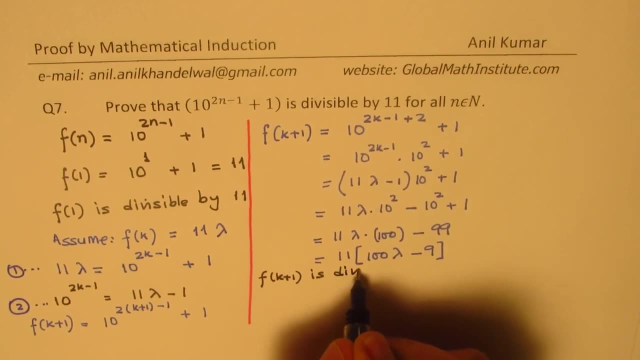 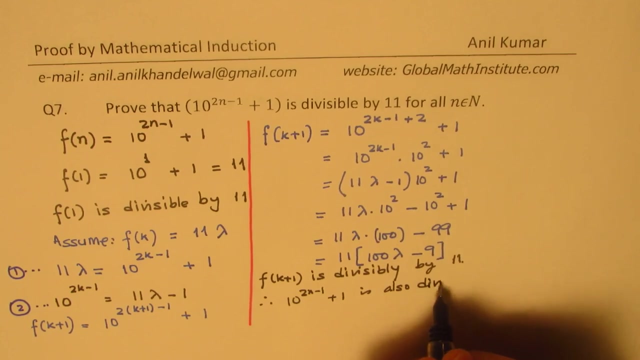 of 11.. So from here we can write down that f of k plus is divisible by 11, and therefore 10 to the power of 2n minus 1 plus 1 is also divisible by 11.. This is using the first principle of induction, right. So this is the application. 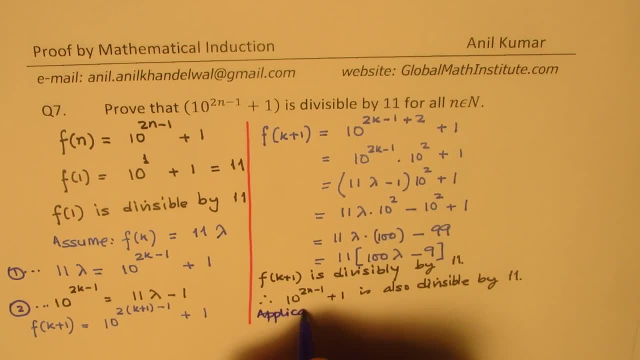 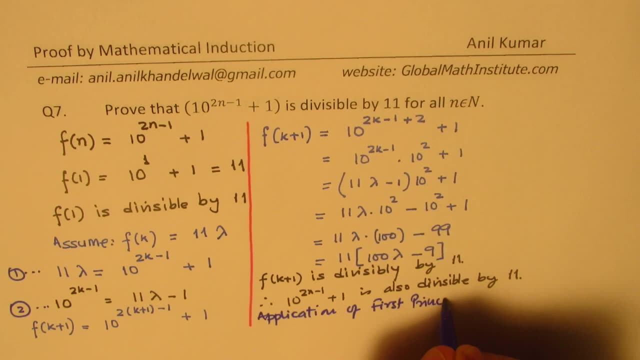 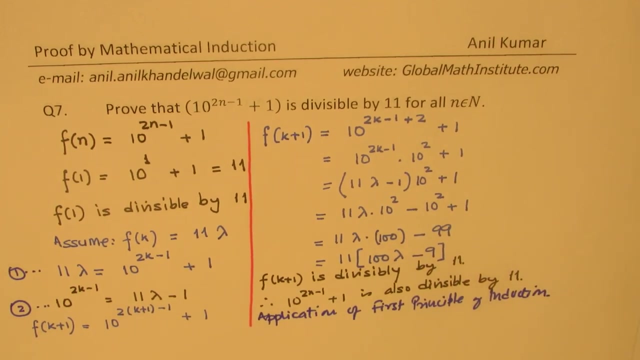 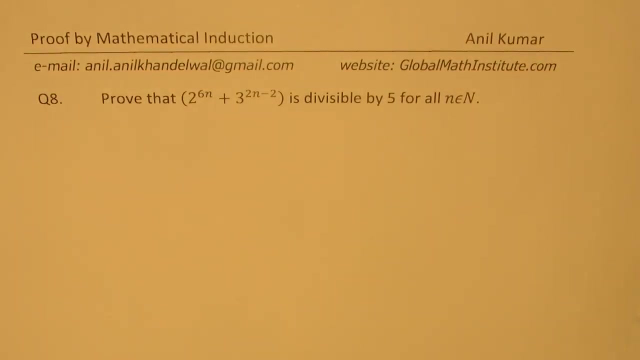 of of first principle of induction. now let's move on and take the last question, which is question number eight for us. you need to now prove that 2 to the power of 6, n plus 3 to the power 2, n minus 2 is divisible by 5 for all values of n. you can always pause the video. 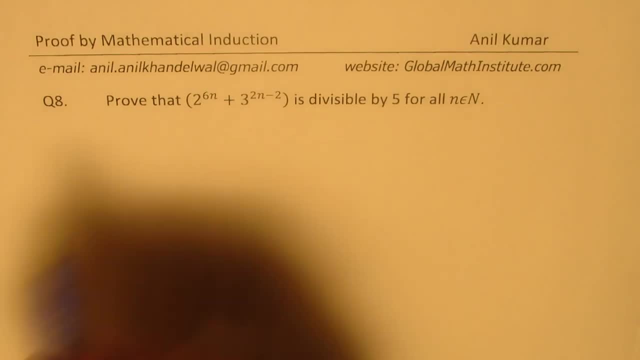 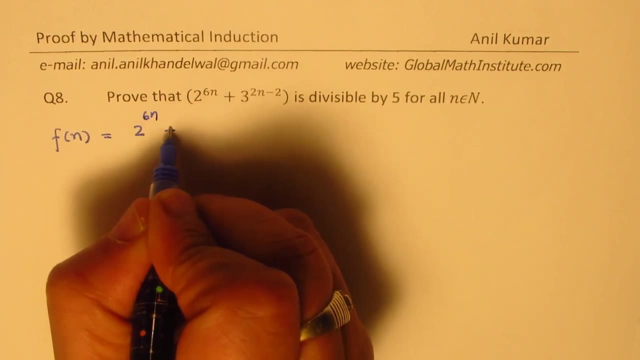 answer this question and then look into my sedations. so we'll define our function f of n as equal to 2 to the power of 6, n plus 3 to the power of 2, n minus 2. so for f of 1, what do? 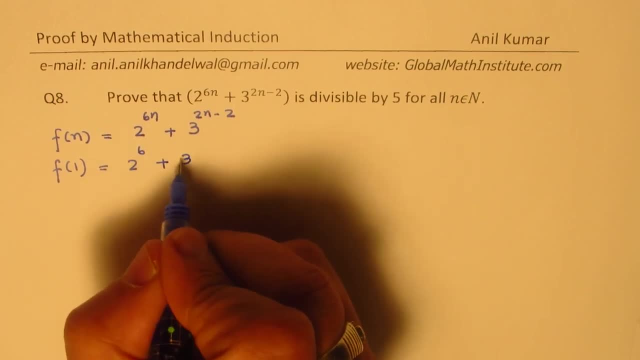 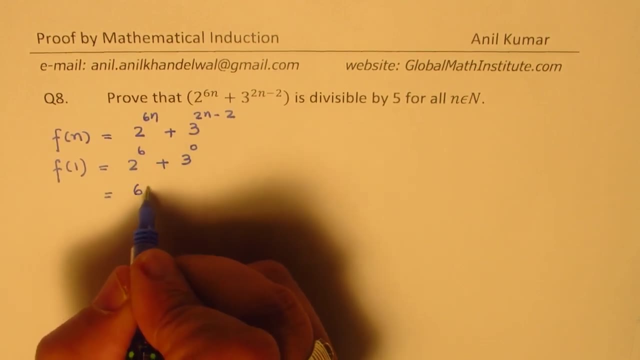 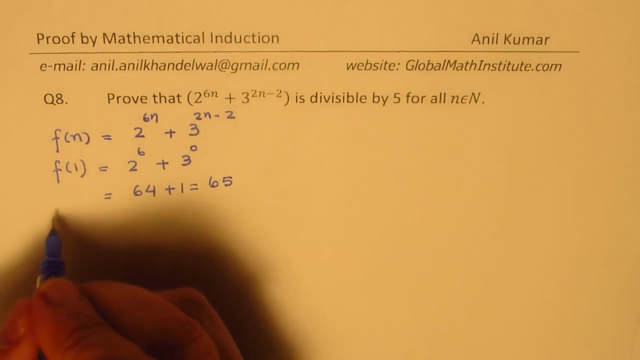 we get. so we get 2 to the power of 6 plus 3 to the power of 0 right. so which is 2 to the power of 6 is 64 plus 1, which is 65. so clearly it is divisible by 5. so we have: 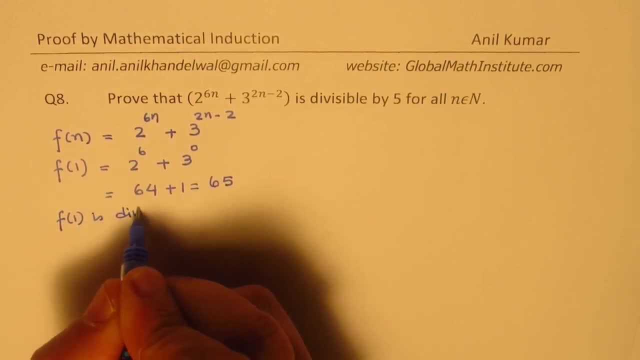 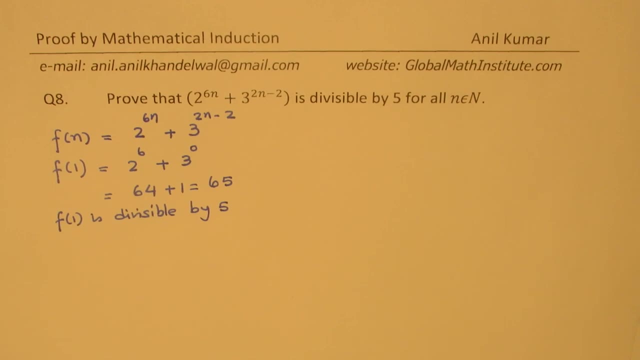 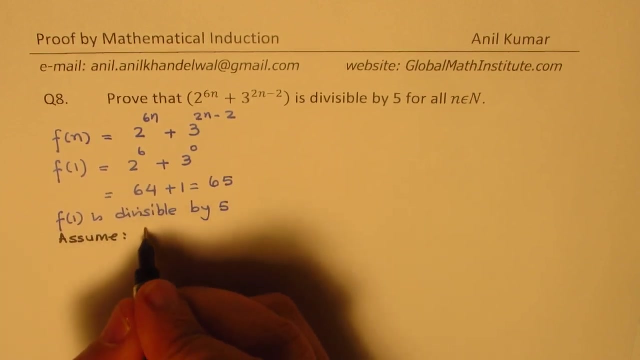 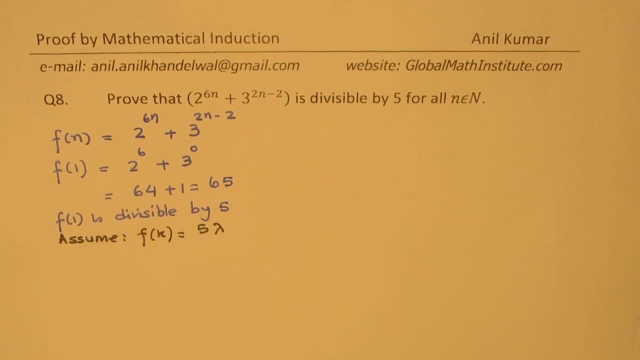 f of 1 is divisible by 5, so that part is true. so now we are going to do an assumption, and our assumption is that f of k is 5. lambda is also divisible by 2, right, so that is our assumption. f of k is a multiple. 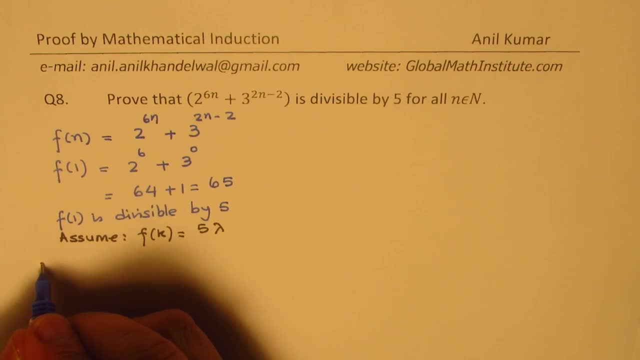 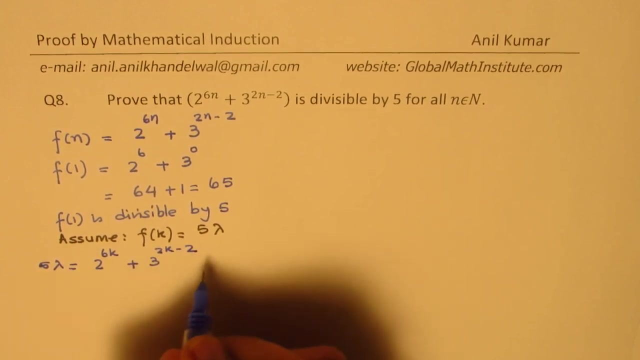 of 5, and what we need to prove is so, basically, we are saying that 5 lambda is equal to: if i write k here, we get 2 to the power of 6 k plus 3 to the power of 2 k minus 2, right, so that is our. 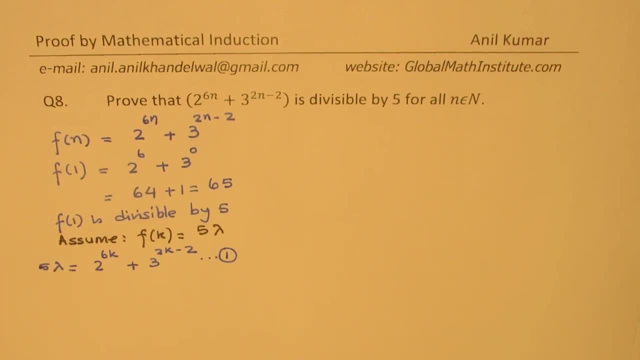 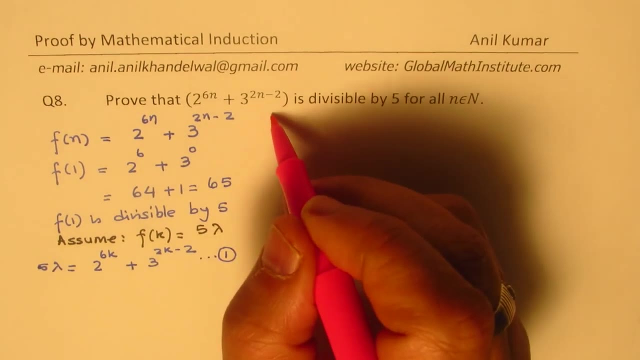 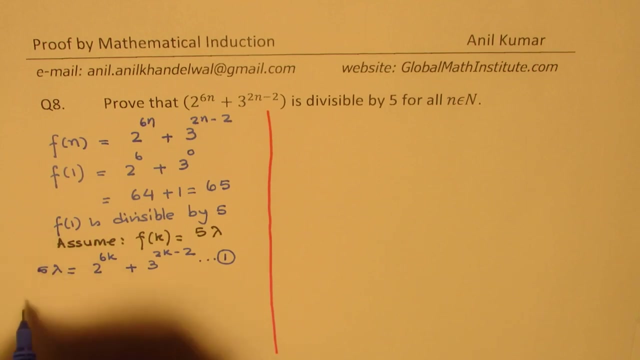 equation number one. so we have different kinds of proofs. you could also rearrange this equation right in different fashion, right? so we'll leave it here. and the idea here is now to find whether f of k plus 1 is a multiple of 5 or not. so k plus 1 will be 2 to the power of 6, k plus 1 plus 3 to the power of 2. 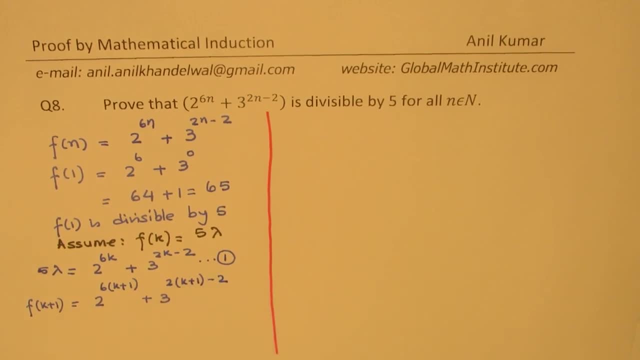 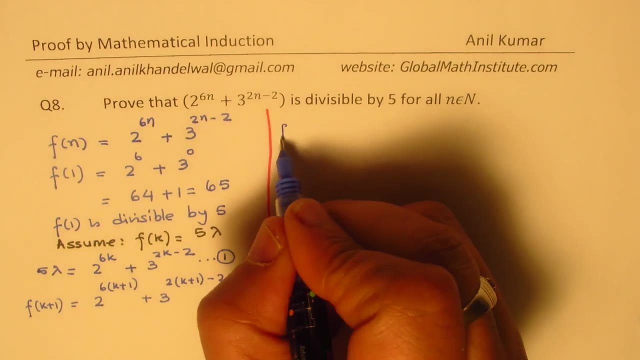 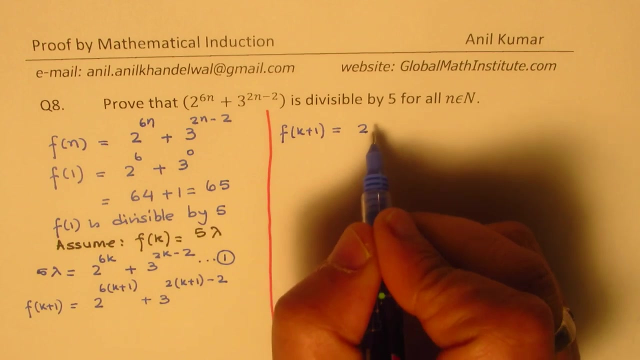 k plus 1 minus 2k. So let's take it to the right side and then solve this. So we get f of k plus 1 as equals to. since we have this form, we write this as 2 to the power. 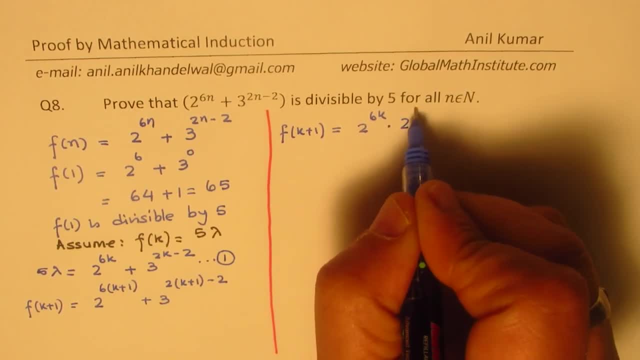 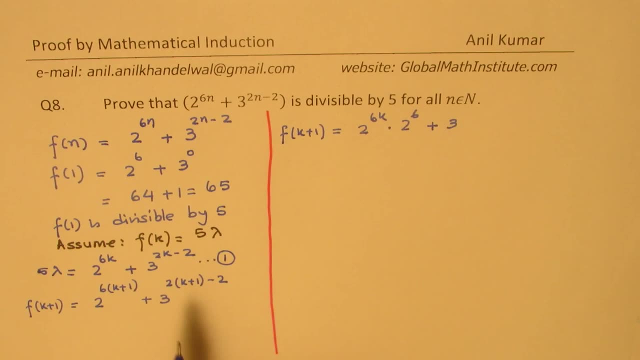 of 6k times 2 to the power of 6, right, And the second term will be 3 to the power of. we should write this as 2k minus 2, right, So we get 2k minus 2 times 3 to the power. 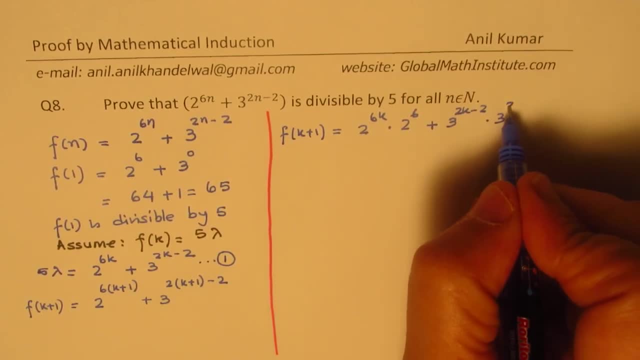 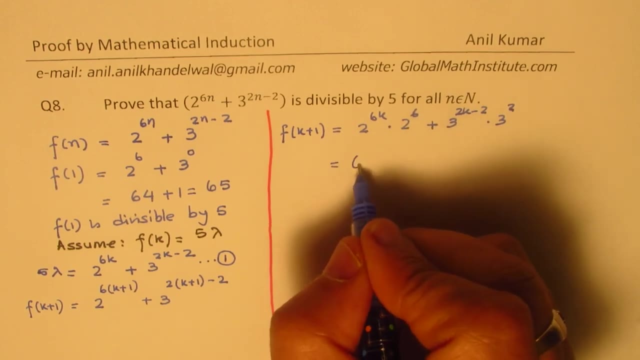 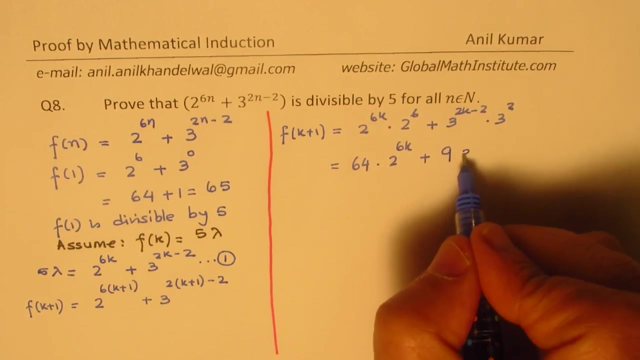 of 2, right, which is 9.. So that is how we can write this. And this, 2 to the power of 6 is 64. So we get 64 times 2 to the power of 6k plus, and that is 9, right, 9 into 3. 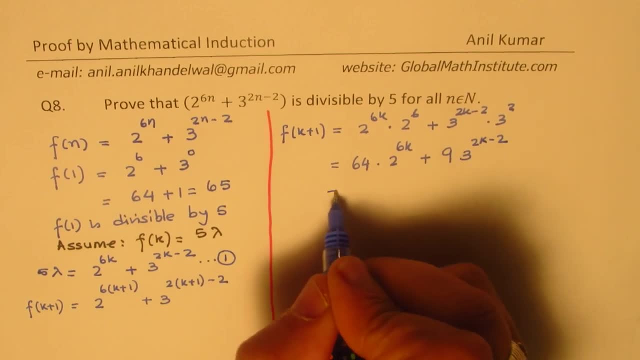 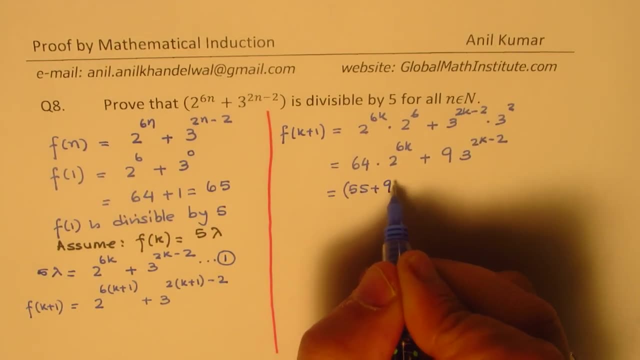 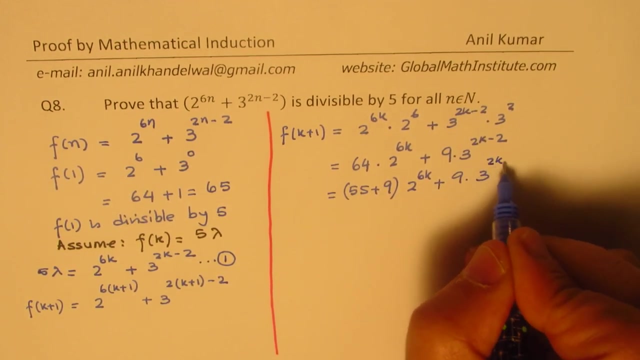 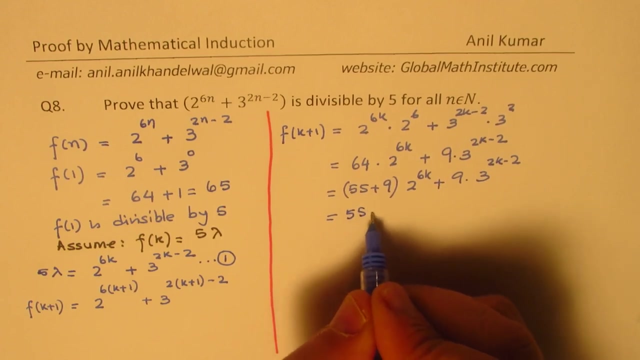 to the power of 2k minus 2.. Now 64.. Okay, So this can be written as 55 plus 9 times 2 to the power of 6k, plus 9 times 3 to the power of 2k minus 2.. And now from here, we can write one term as 55, which is a multiple. 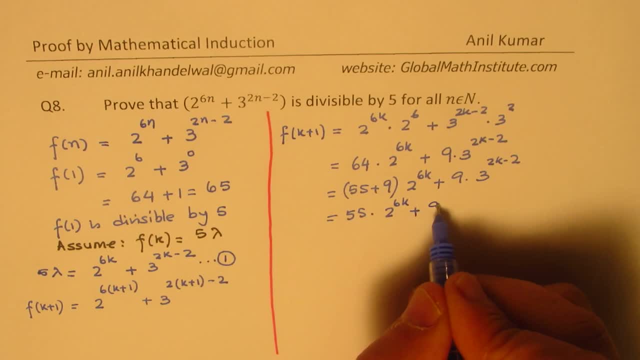 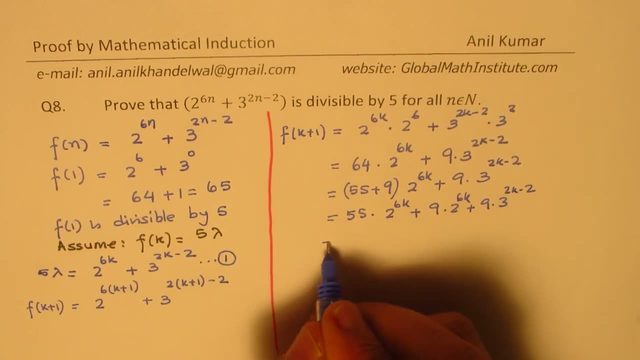 of 5, times 2 to the power of 6k, plus 9 times 2 to the power of 6k, plus 9 times 3 to the power of 2k minus 2.. So what we get here is 55 times 2 to the power of 6k plus 9 comma. 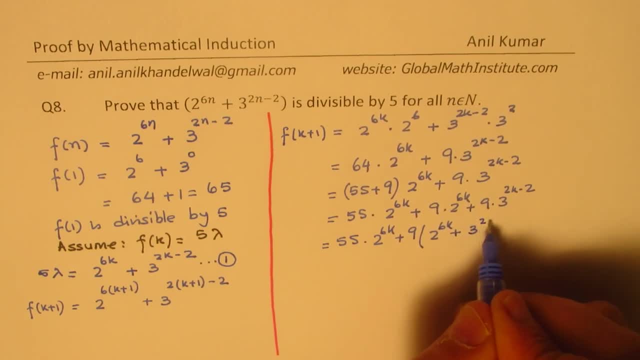 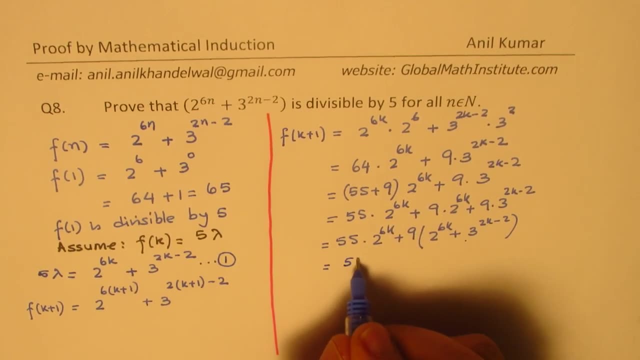 So we get 2 to the power of 6k plus 3 to the power of 2k minus 2.. Now this term here is 5 lambda, So we can write this as 55 times 2 to the power of 6k plus 9 times 5 lambda. 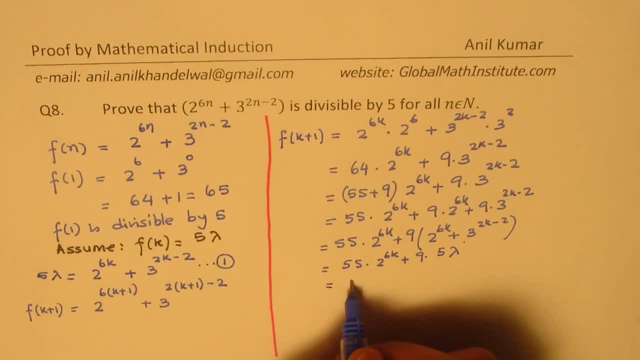 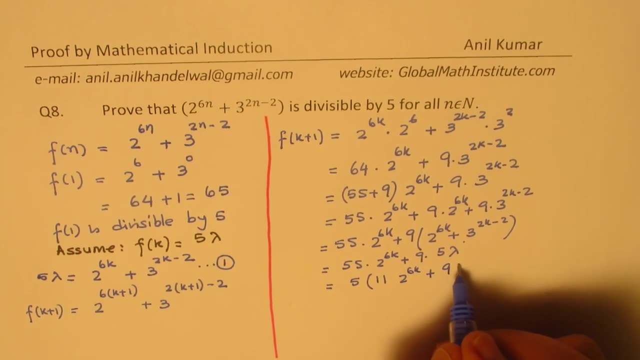 So 5 is a common factor And what we get here is 5 times 2 to the power of 6k plus 9 times 2 to the power of 6k plus 9 lambda. Is that clear? So clearly we have shown that f of